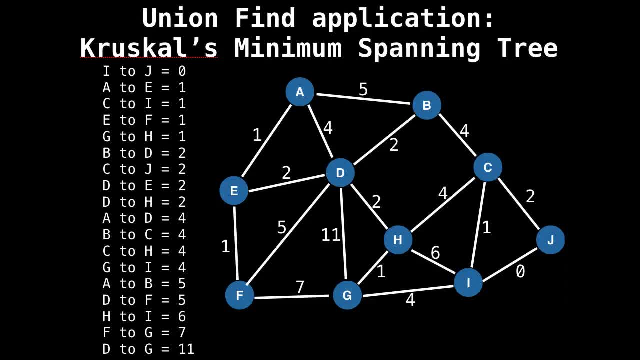 order. So next we're going to start processing the edges, one at a time. started starting with the top, so i to j. So I've highlighted the edge i to j in orange And you can see that it connects nodes i and j. i and j currently don't belong to any group, so I'm going to. 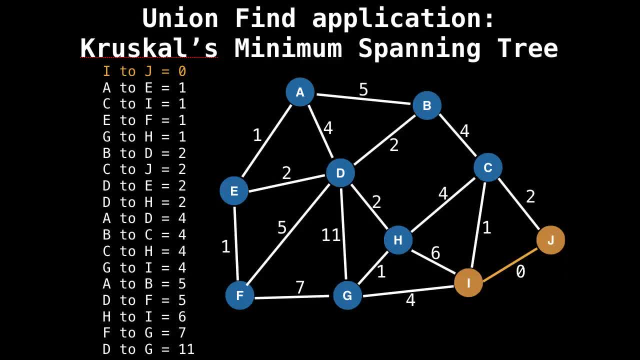 unify them together into group orange. Next is edge: a to e. So a to e don't belong to any group, so I'm going to unify them together into group purple. Next is c to i. So i belongs to group orange, But c doesn't have a group yet, so c can go into group orange. Alright. e to. 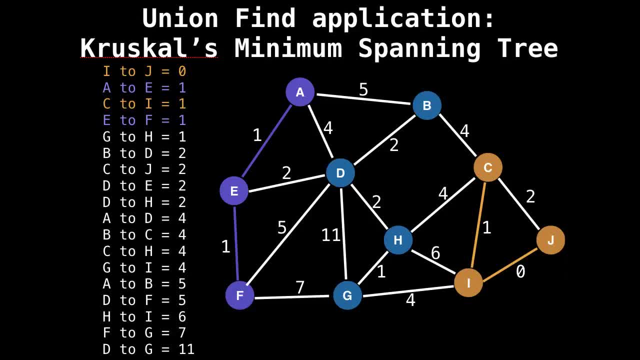 f. f doesn't belong to group, so f can go to group purple. Next h and g. Neither h nor g belong to a group, so I'm going to say you guys belong to the red group. Next we have a, d to b. They also don't belong to a. 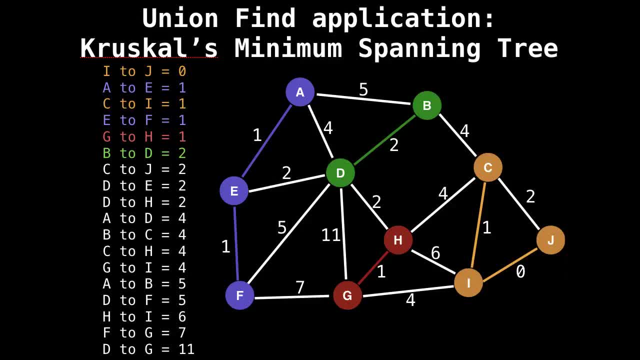 group. So give them their own group, let's say group green. Alright, and now- I believe this is when things start to get interesting. Now we're trying to connect C to J, But notice that C and J are a. both belong to group orange. So we don't want to include that edge because 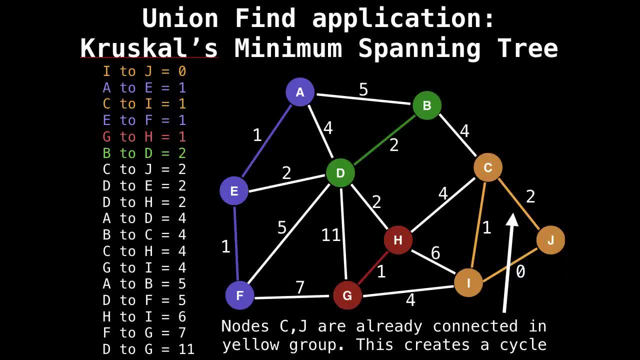 it's going to create a cycle, So ignore it. And to check that they belong to the same group, we would use the find operation in our union find to check where group they belong to. So this is when the union find really comes into play. Next is edge D to E. So 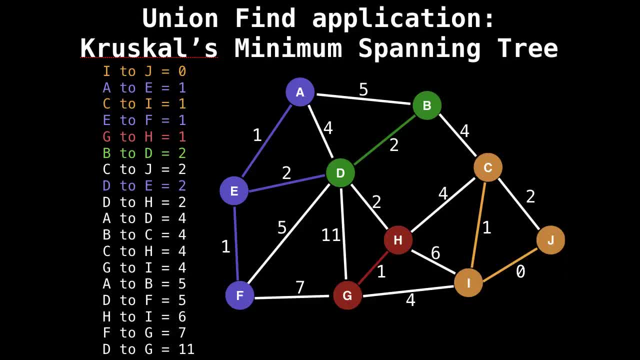 note that he belongs to purple and D belongs to group green. So now we want to merge them together because they don't belong to the same group. So either the purple groups want to become the green group, their green groups have to be the purple group.